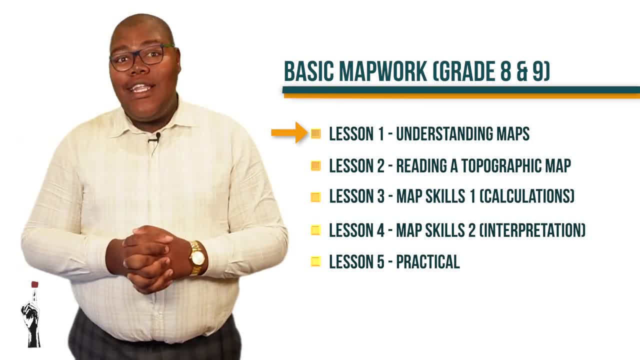 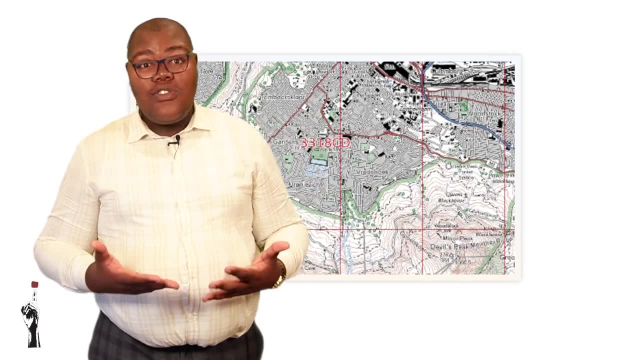 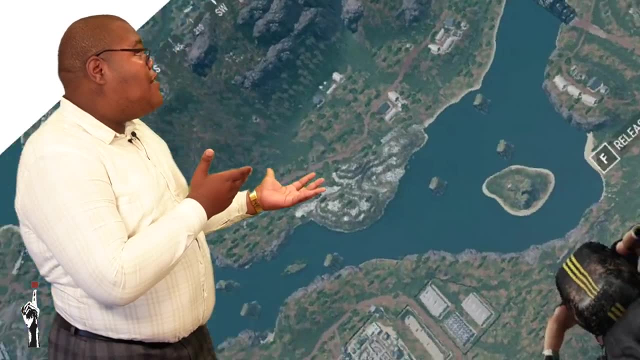 happy to be doing this lesson for you. Welcome to my Tumamina teaching. Maps are awesome. If a picture is worth a thousand words, maps are worth 10,000 more. They are jam-packed with loads of information. Excuse me, editor, the last lesson should have not been there. They are part. 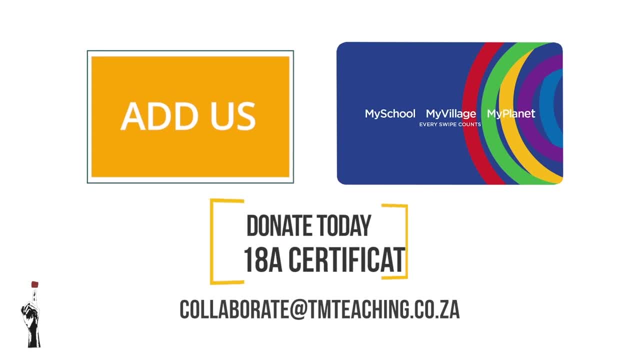 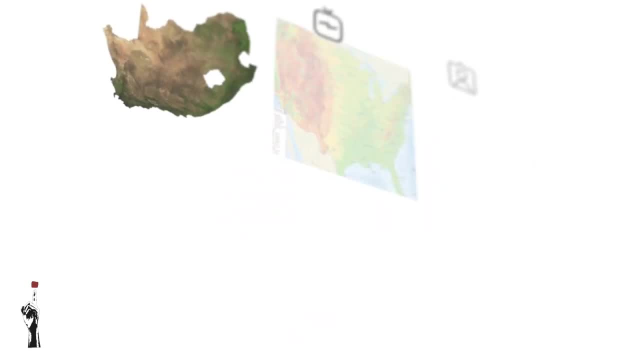 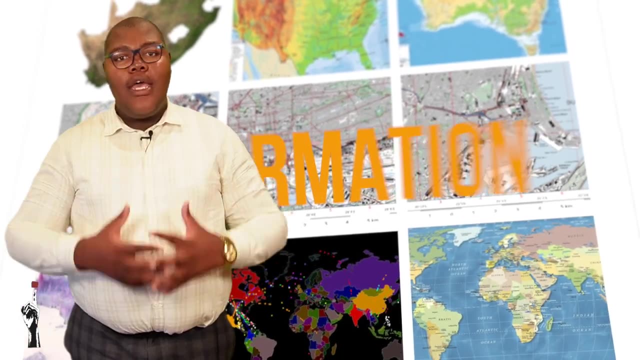 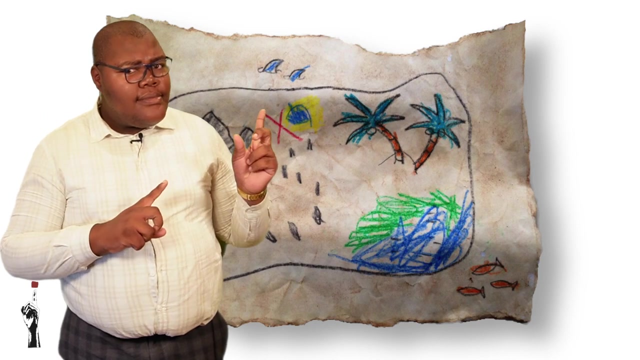 of a game. Today, we'll be learning about the fundamentals of maps as well as learning about maps. Maps are about conveying all types of information in a straightforward and visual way. Do you remember when you were a kid and you played around with treasure maps? What did they give you? 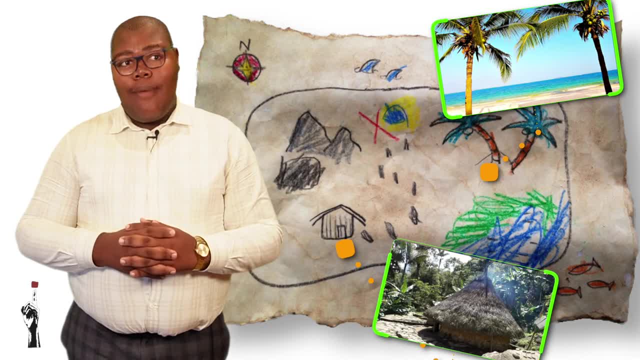 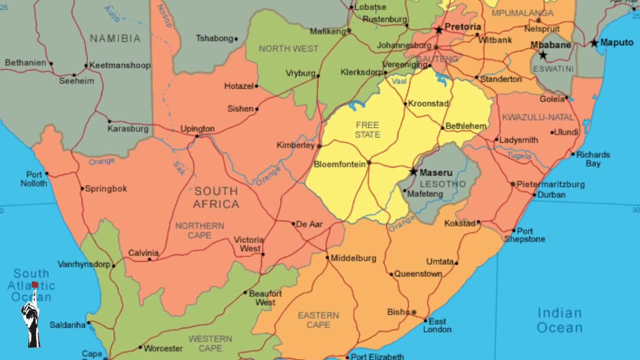 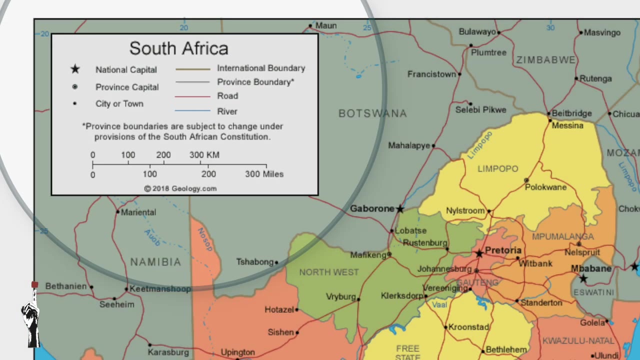 Information right. So do maps for grown-ups. They give all types of information. They teach about the world by displaying country sizes. They can give us the area which is the area of the country and forms and locations of geographic features, So, for example, where the mountains are. 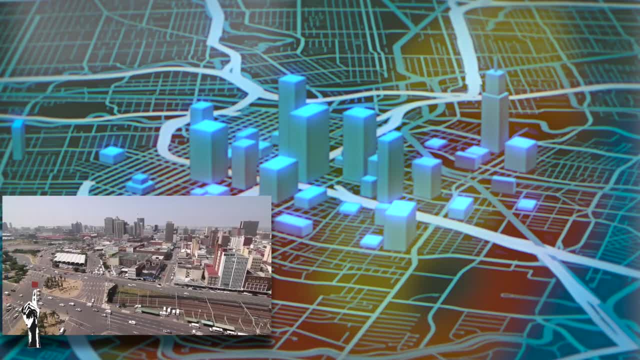 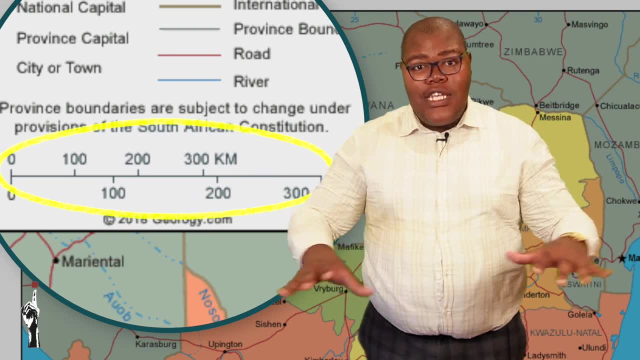 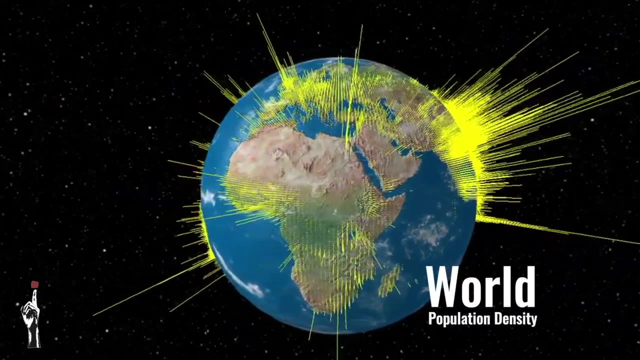 where the rivers are and where buildings are, et cetera, And distances between places. So these distances are generally scaled down to fit into a sheet of paper. Maps can depict the distribution of objects on earth, So we are able to tell sediment patterns from the earth. So when you're 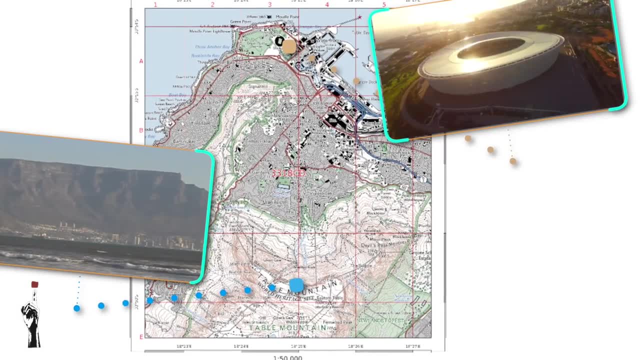 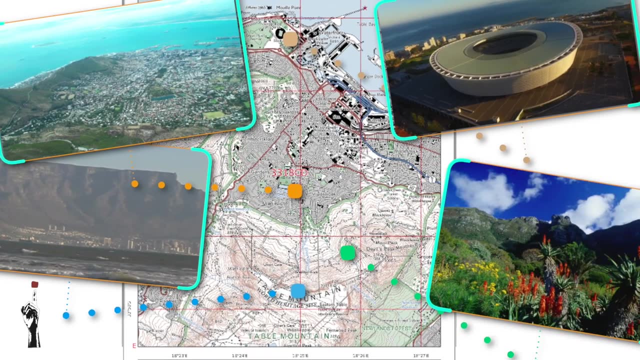 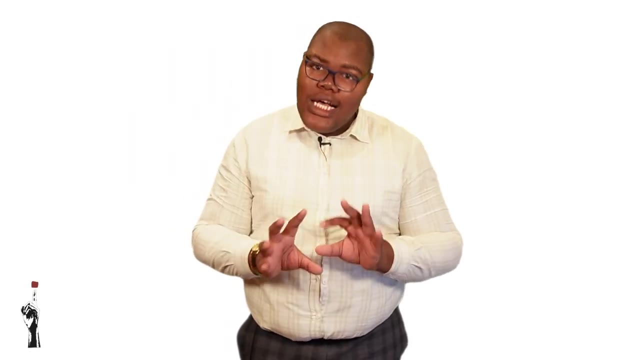 in grade 10,, 11 and 12, you'll learn about different sediment patterns Right. They can tell us where most people are concentrated and which areas have the most vegetation. There are many reasons why maps are so important, And I think that they are worth a. 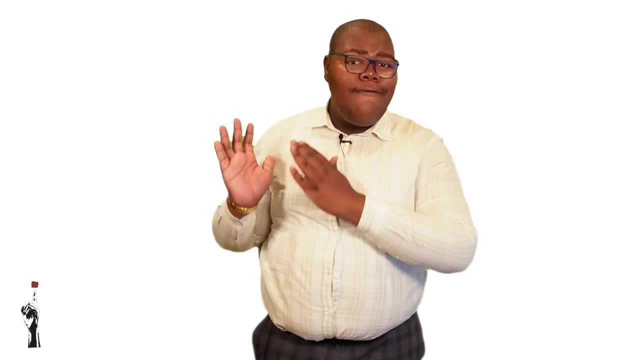 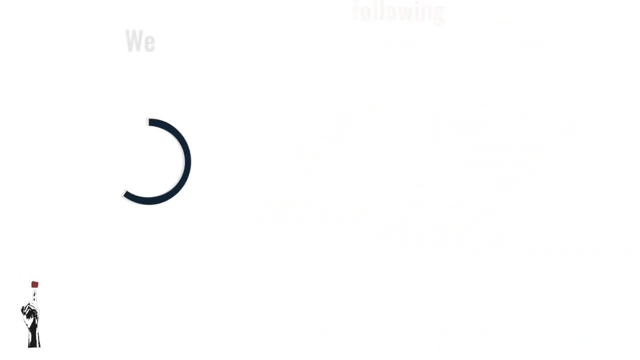 class discussion. So if you're in class, right, I'm going to have four headings pop up on the screen and you're welcome to just take a quick pause to discuss some of the headings that come up. In this lesson, we'll introduce the following maps: A physical map. 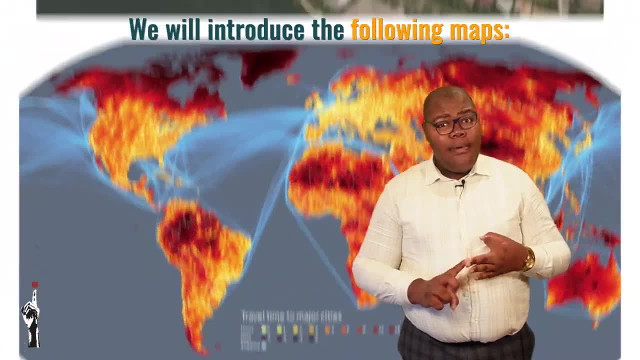 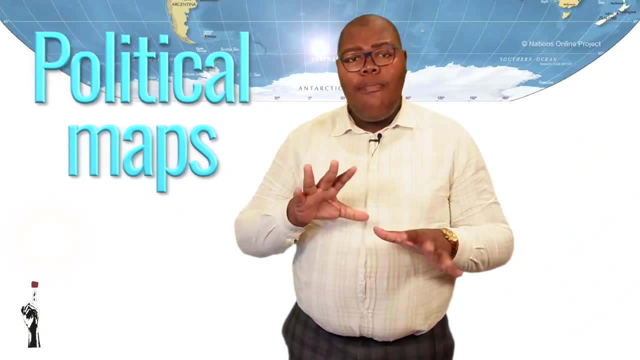 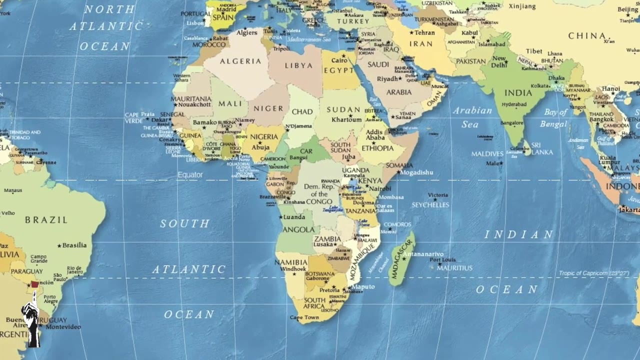 a political map, a thematic map, an author photo and a topographical map. Let's start off with the political map. A political map is a map that looks like the one I have here. We can use political maps, as I said earlier on, to depict different types of information We can. 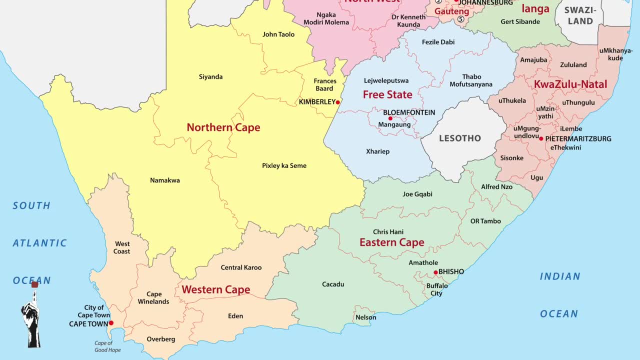 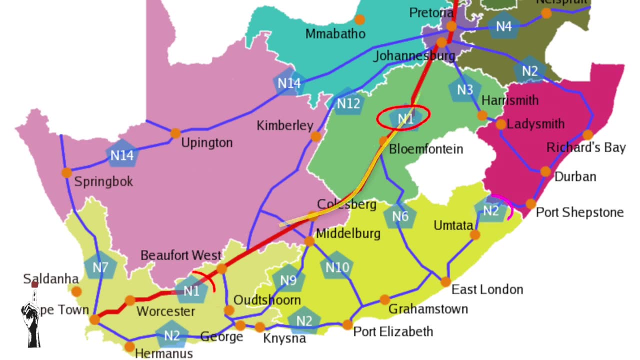 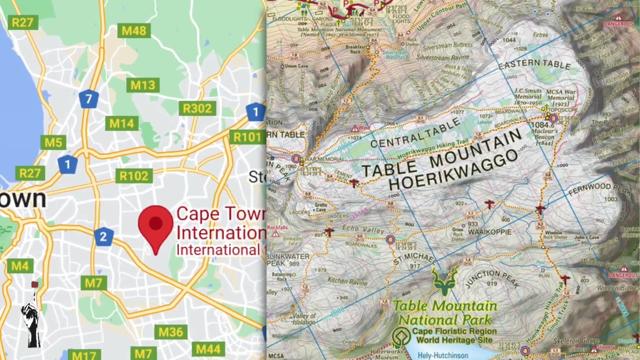 depict borders of countries. We can look at provincial boundaries. We can look at capital cities and other important towns. We can have major roads like the N1 and N2 in Cape Town. We can have airports or other special and significant places. Political maps show legal jurisdictional. 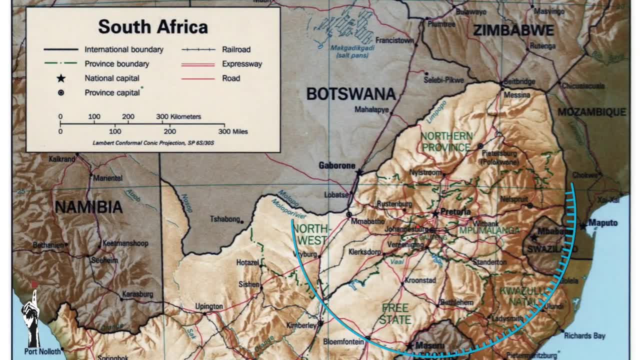 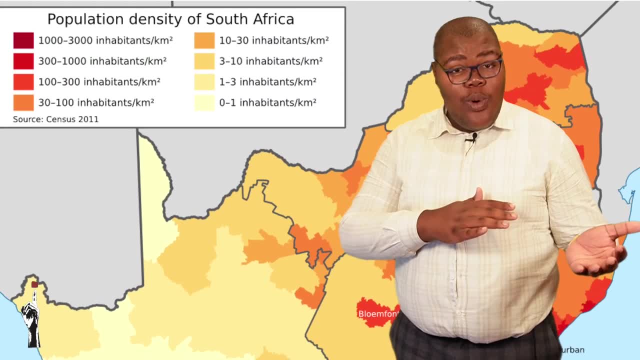 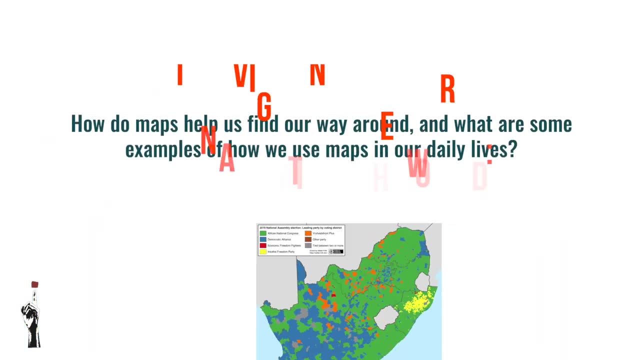 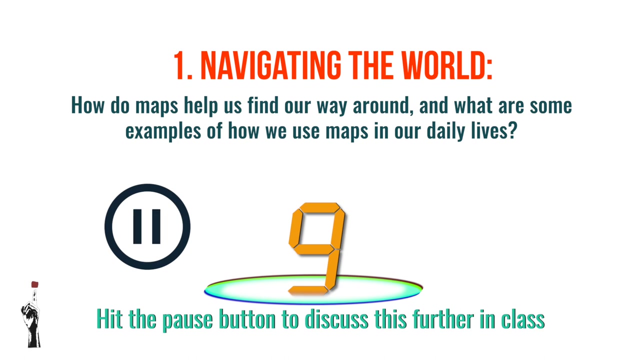 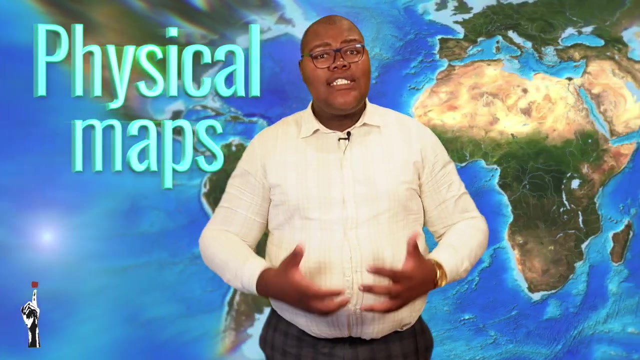 political or administrative boundaries. These help people understand the geography of the world. These maps are frequently used to depict census data, like the one we had in 2022, and even election results, like the ones we're having in 2024.. Now we're transitioning from political maps, going into physical maps. Physical maps depict: 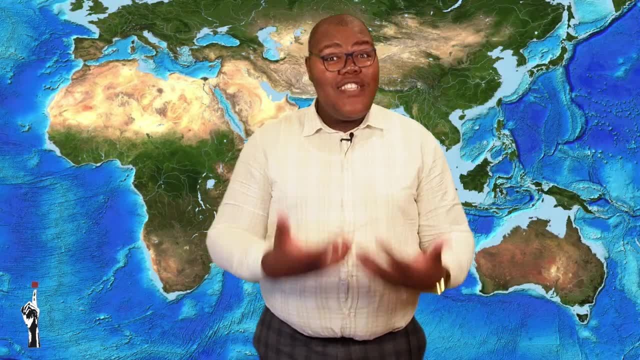 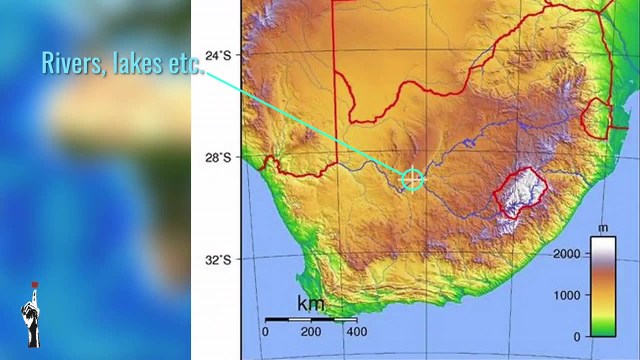 the natural features of the earth. So the things we have present in the world of today are 팍 temple on either side of the В quatro Havens of the Earth. we see physically that come from the earth. We can use physical maps to see rivers, lakes. 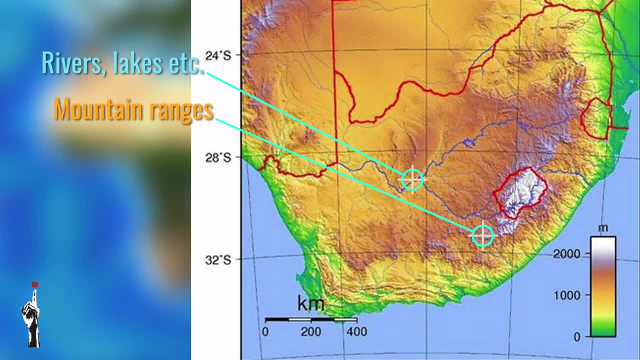 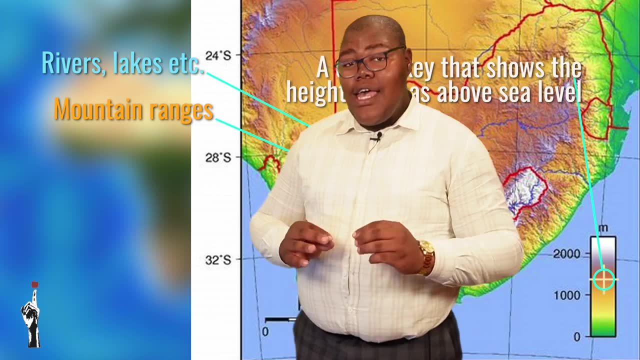 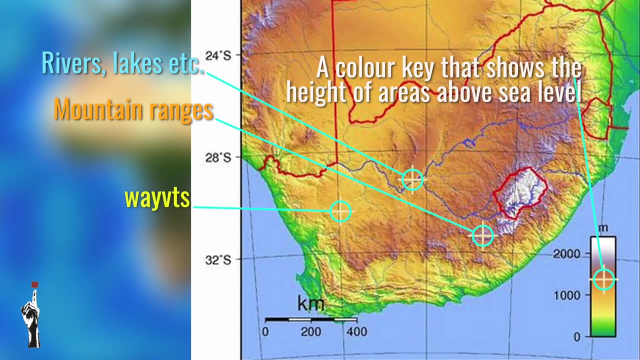 and other water bodies. We're also able to see mountain ranges right. It also has a colour key that shows the height of areas above sea level. Remember that our zero in maps is sea level, not zero metres. We can also see deserts, marshes, swamps and deltas from a physical map. 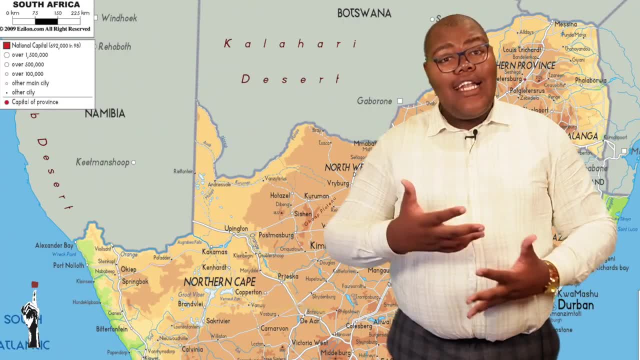 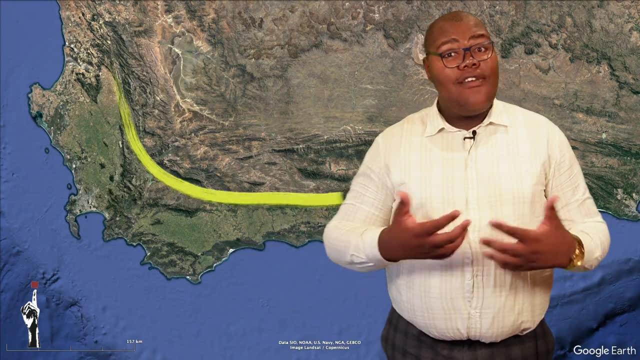 Physical maps are useful for studying the natural environment and understanding how physical features interact with one another. For example, we're able to see how mountain ranges affect the weather. Do you remember in climatology grade 8, you learnt about autographic grain. We are able. 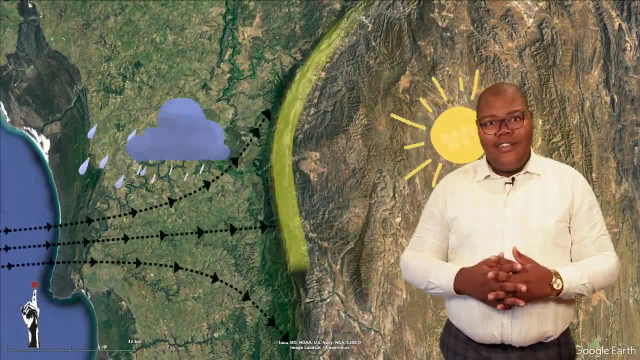 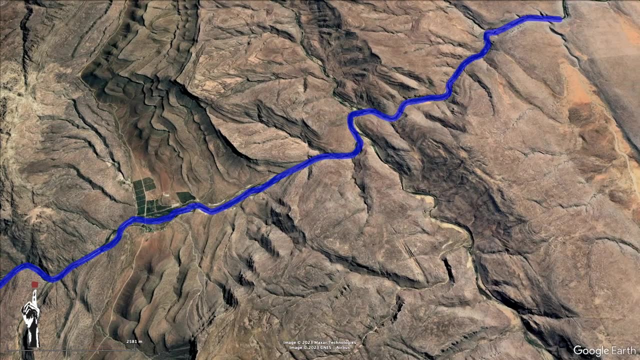 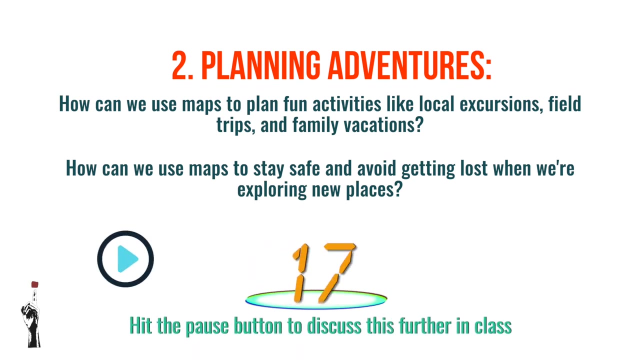 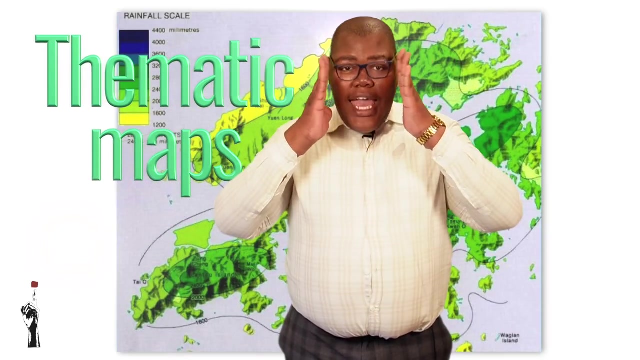 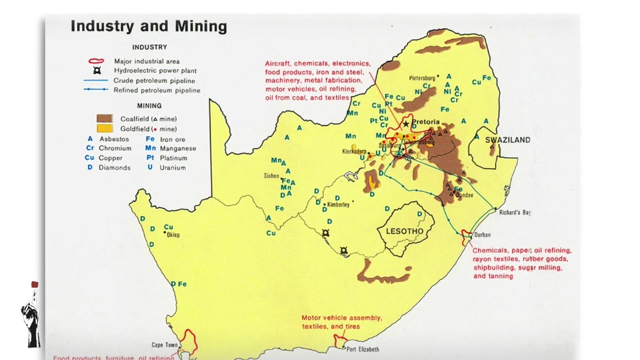 to see if an area gets the same amount of rain as the other. We can also see how the rivers shape the landscape on which they flow. And now we're transitioning to thematic maps. The thematic maps display data about a specific theme or topic. The thematic maps look like the one I have here. They are able to give us. 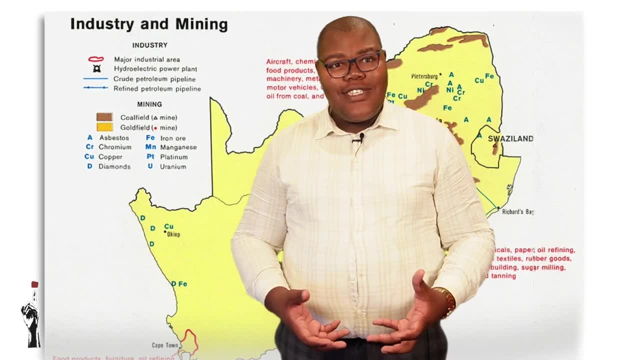 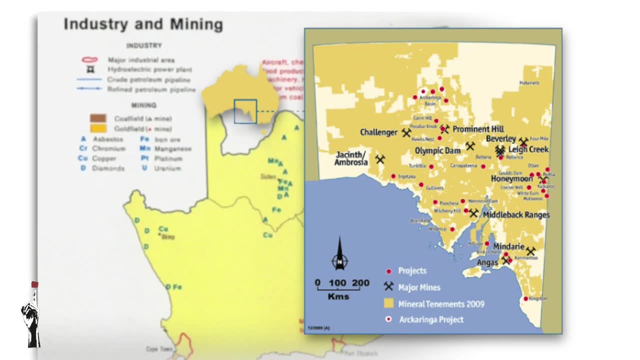 information about specific land uses and resources. The thematic maps can use small images of symbols to express some of these concepts, such as minerals and mines. They can also show us industries and power stations. We can also see how the rivers shape the landscape on which they flow. 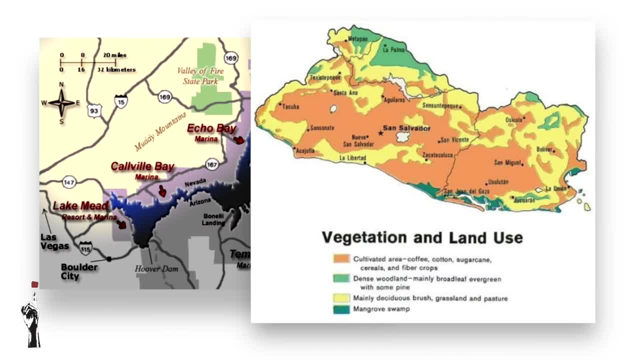 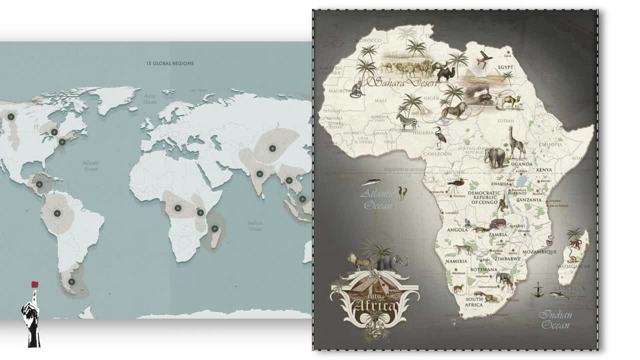 They can also show transport routes and areas where a particular crop is farmed. They can also show us areas where a particular type of animal is farmed. The thematic maps are quite powerful. They can be used to analyse different spatial patterns and relationships between different 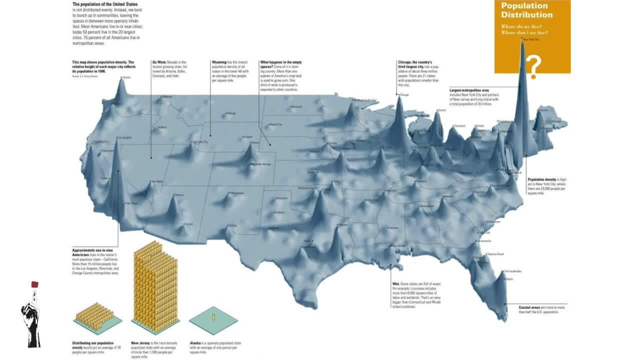 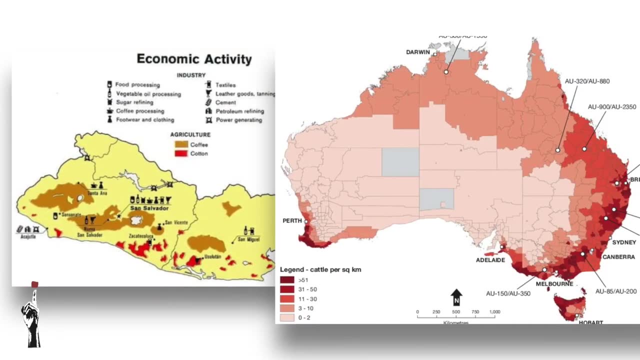 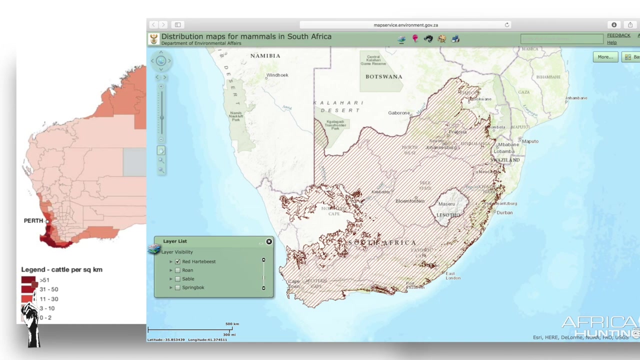 phenomena such as the relationship between population density and urban development or the distribution of natural resources across a region. These maps can also be used to study the impact of urban activities on the environment, such as the distribution of pollution sources or even the location of wildlife habitats. 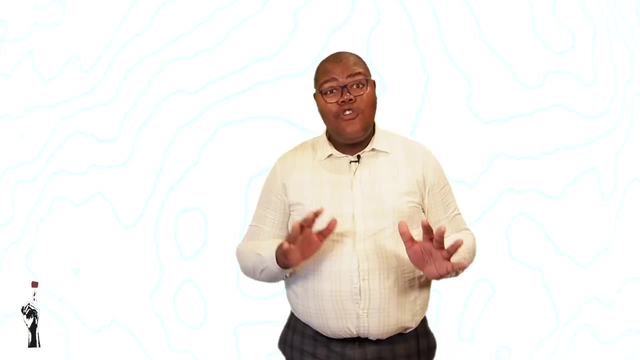 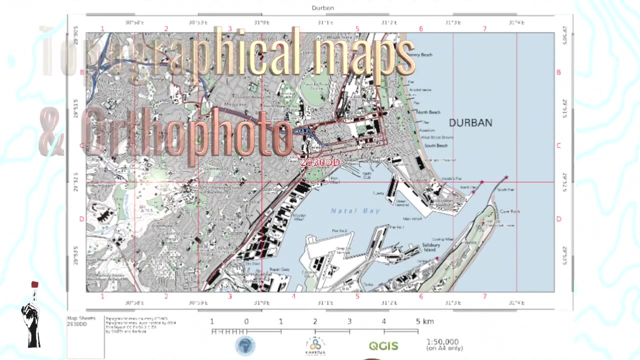 And now Grade 8s and 9s, we are moving to the two maps that are most important for your high school career: topographical maps and orthophotos. A topographical map is a map that shows all the man-made and natural features. 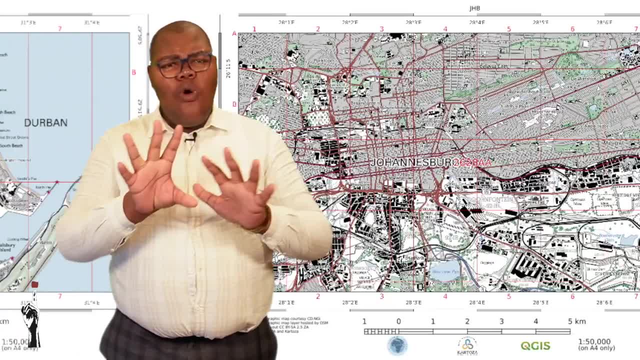 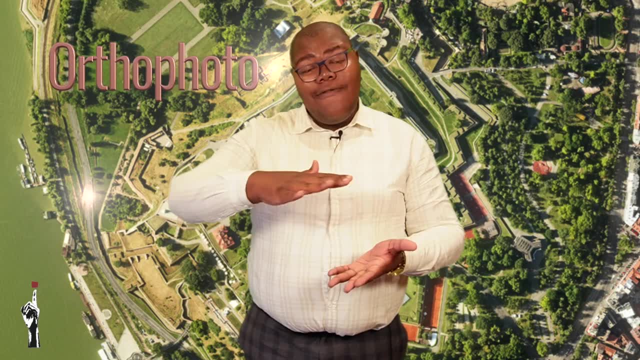 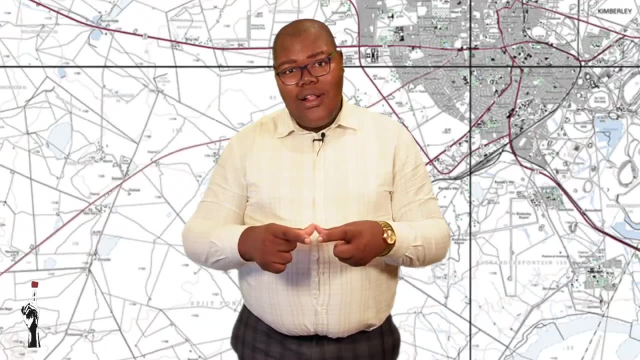 like the one we have right here. We will go into more detail in our next lesson about this map. An orthophoto map is a combination of an aerial photo, which is a photo normally taken by a man, and a map. This map normally covers a small section of a topographical map. That section 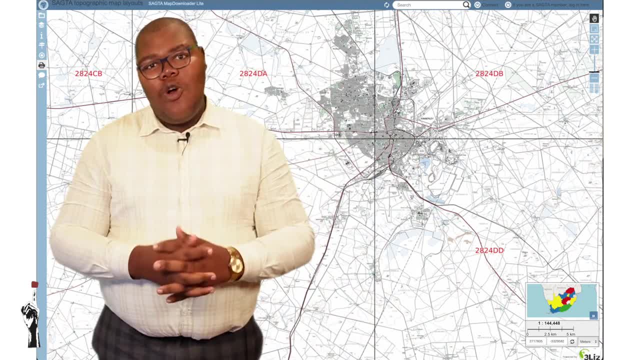 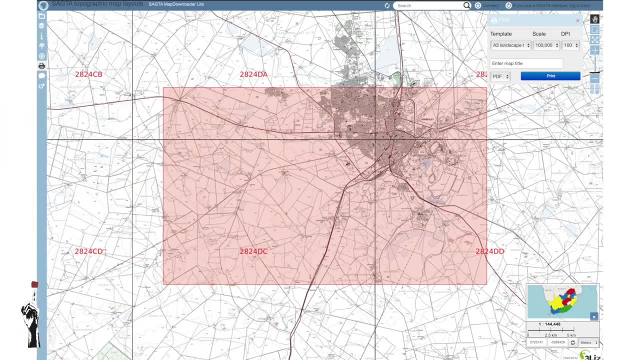 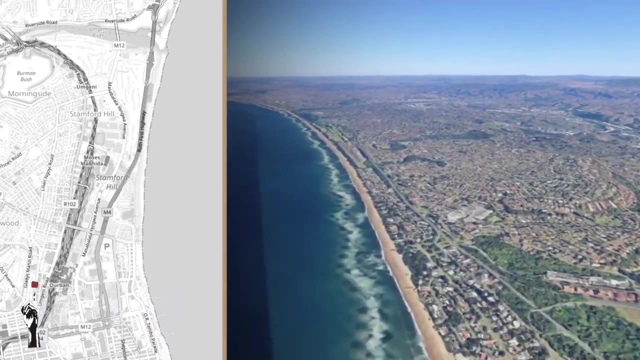 is normally written as a demarcated area within a topographical map. It is normally drawn with a little red square on your topographical map. Okay, learners, now for you to make sense of these maps. On your left is the map and on the right is the VR pilot who will travel through this mapped area to show. 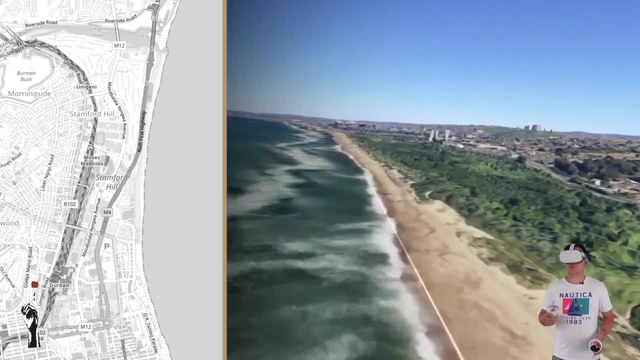 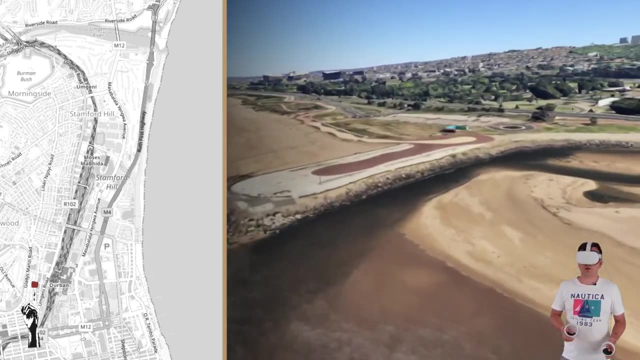 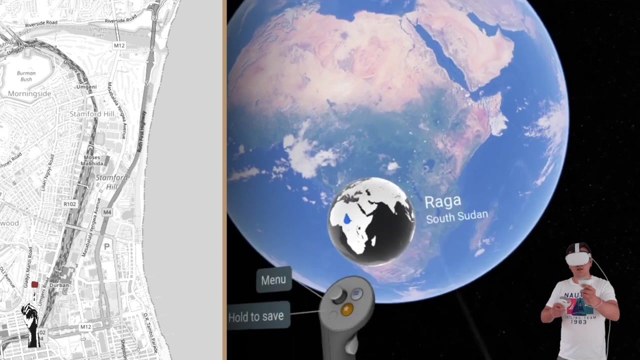 you the areas and features that are represented on the map and hopefully this will help you conceptualize it. I always wanted to go to Durban. Leo, please take us through Durban. Thanks, this is your captain speaking. I'll gladly head over to Durban. 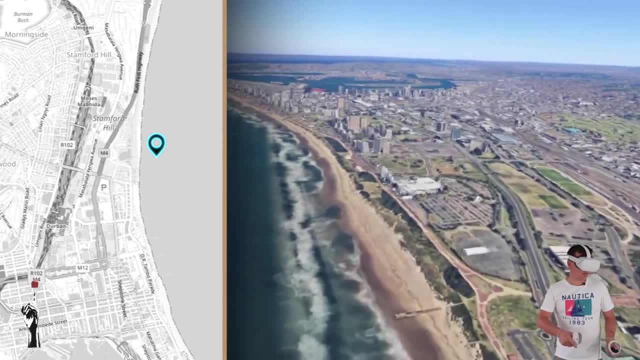 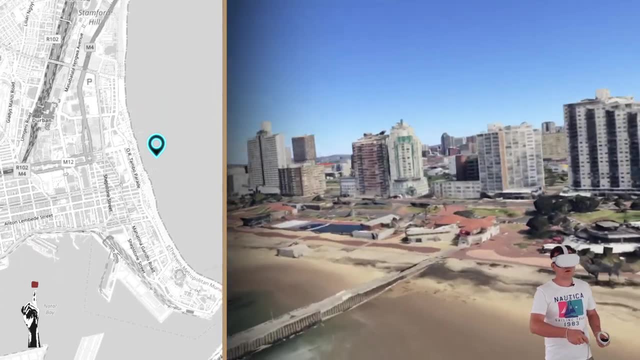 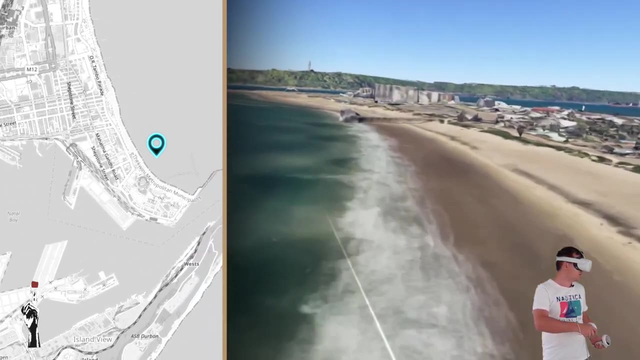 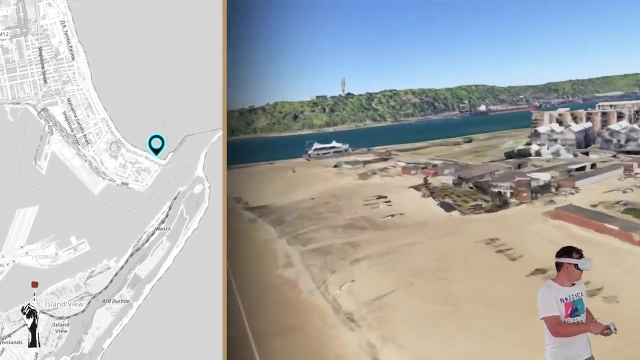 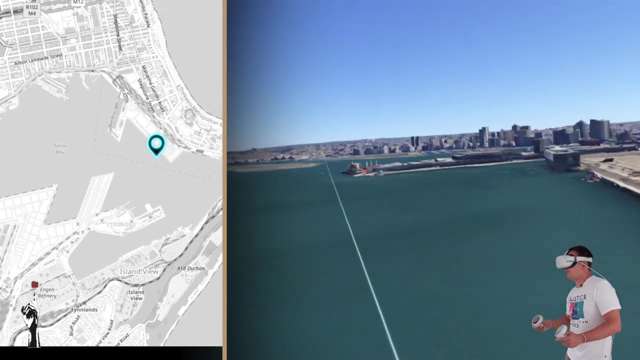 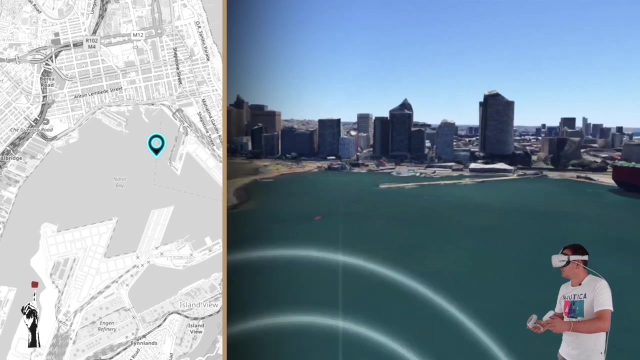 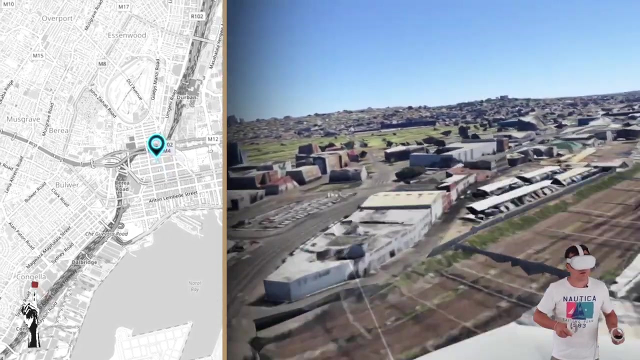 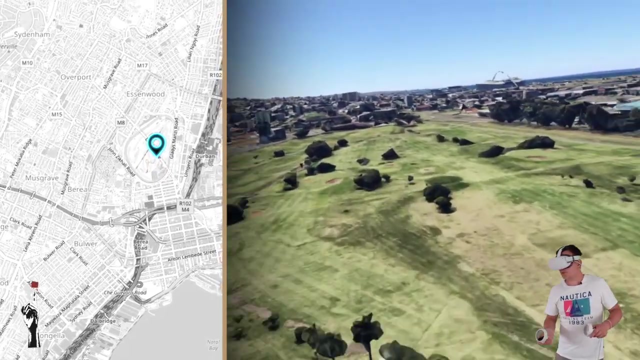 Now, as I fly through Durban, try to identify me on the map and compare the map with the simulations that you see in this fly-through. Can you identify this place? Yeah, I'm covered at this moment. Now we've got a golf course. 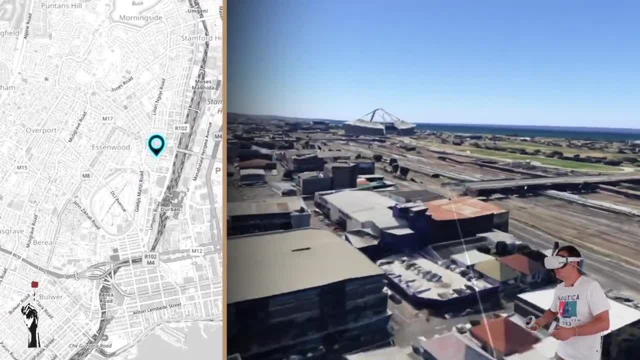 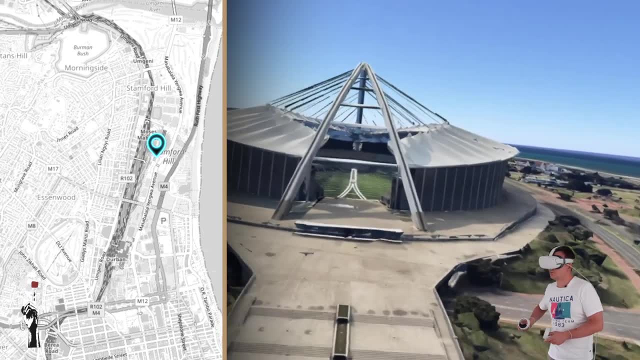 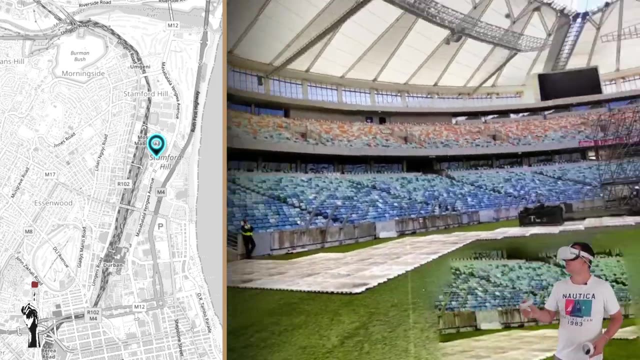 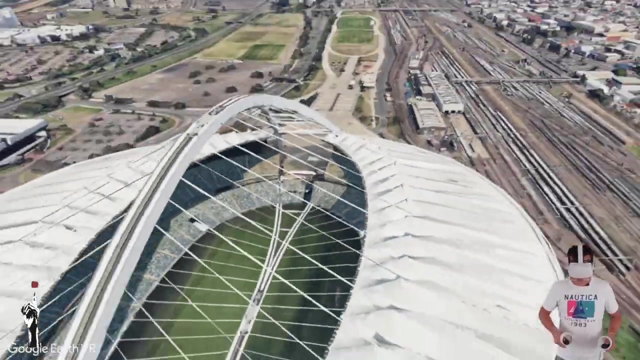 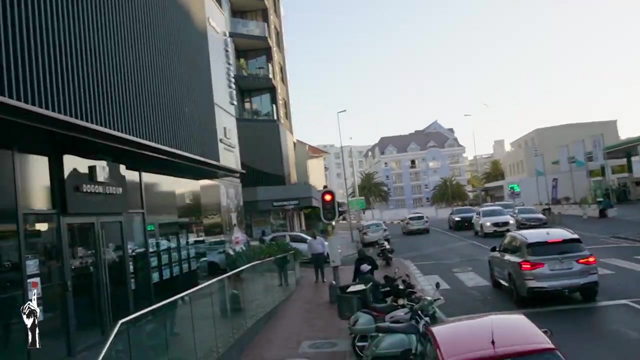 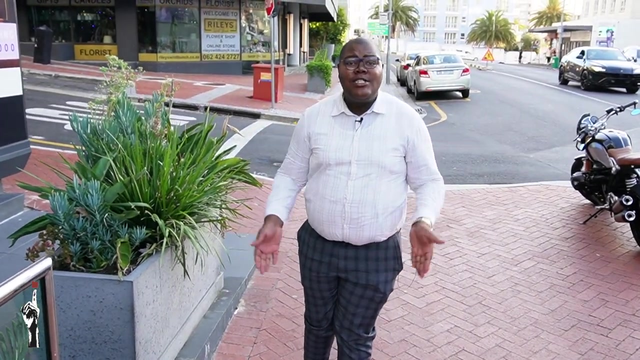 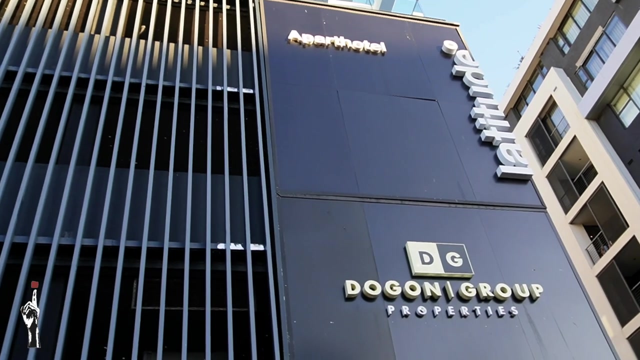 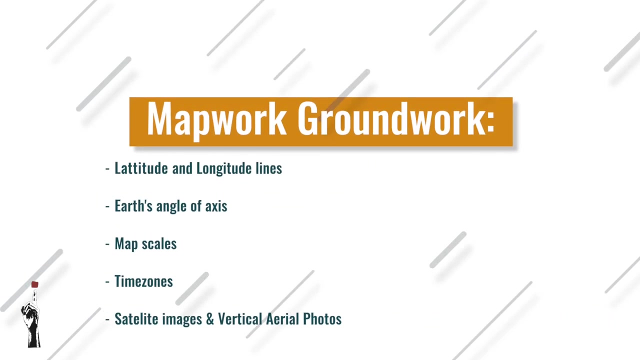 and let's head over to an end. at the stadium. Maps can be used to give our absolute location using latitude and longitude. Guess what? This video happens to be sponsored by the Latitude Hotel in Cape Town. Now I'm going to run through some of the basics of map work that are very important. 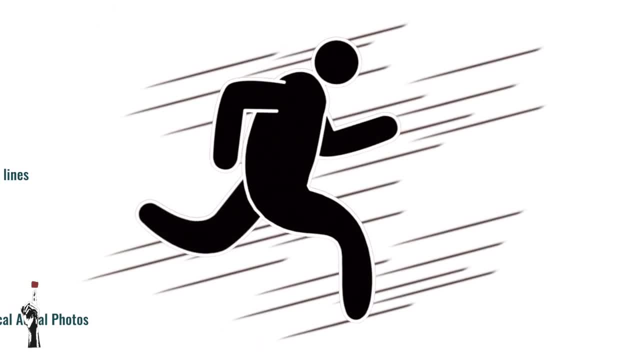 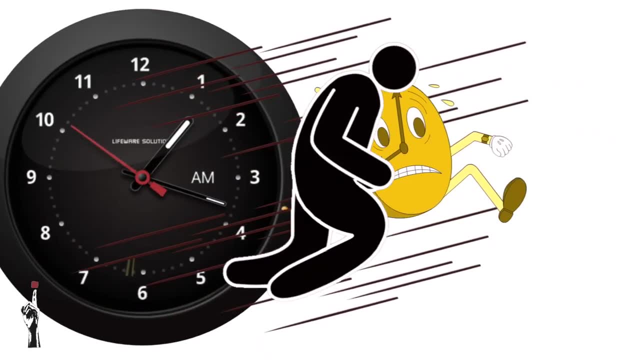 to understand before going into detail about maps. I'll be doing this in great speed, so be sure to watch it again if you missed it the first time. I'm going to cover this list in less than 90 seconds, so let's do it. 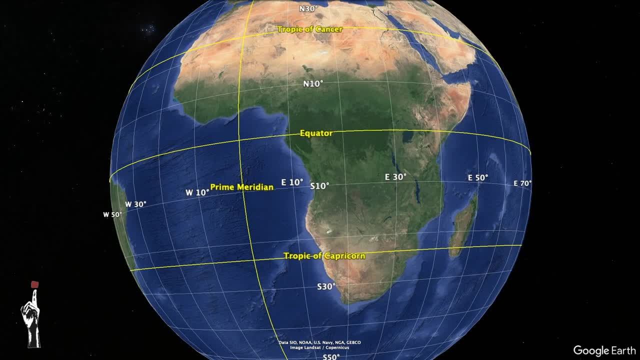 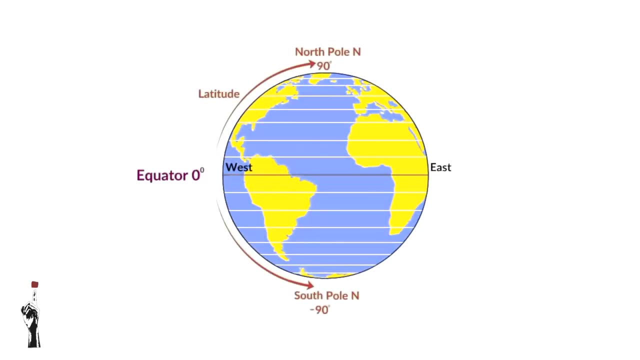 Firstly, latitude and longitude lines are used to help locate points on the Earth's surface. Latitude lines run horizontally around the globe and are measured in degrees north or south of the equator. Longitude lines run vertically and are measured in degrees east or west of the prime meridian. 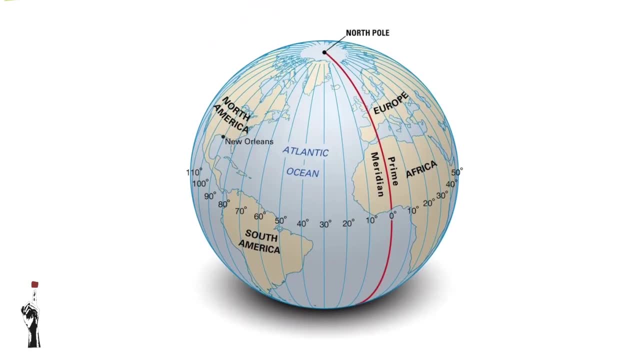 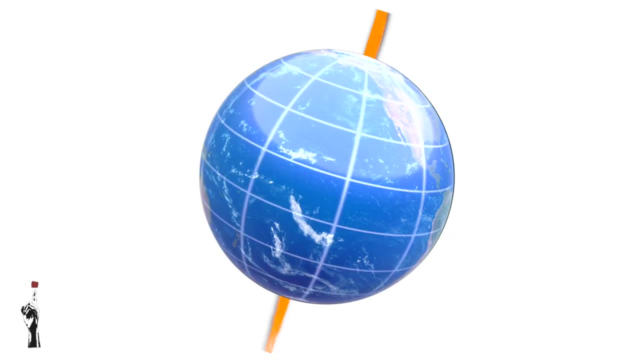 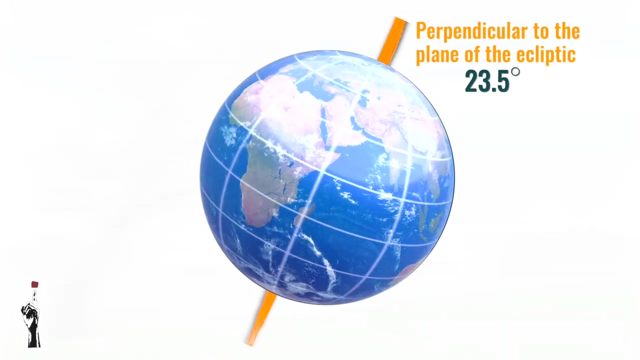 or greenwich meridian, depending on how your primary school teacher called it. In addition, we have the Earth's angle of axis, which is the angle between the Earth's rotational axis and a line perpendicular to the plane of the ecliptic. This angle is currently about 23.5 degrees, which is why we have the seasons on Earth. 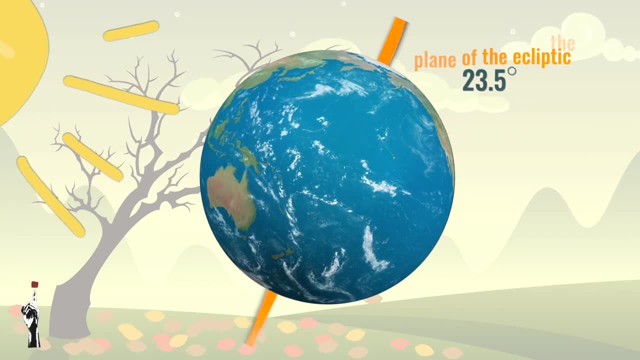 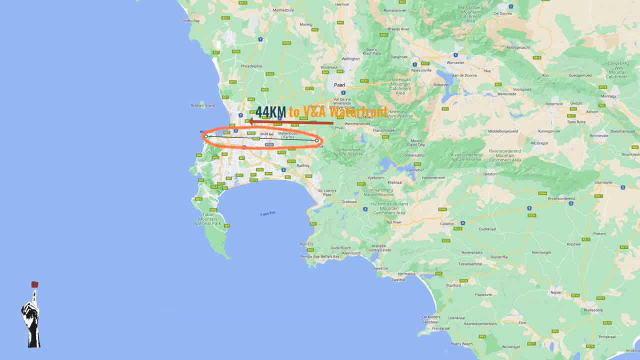 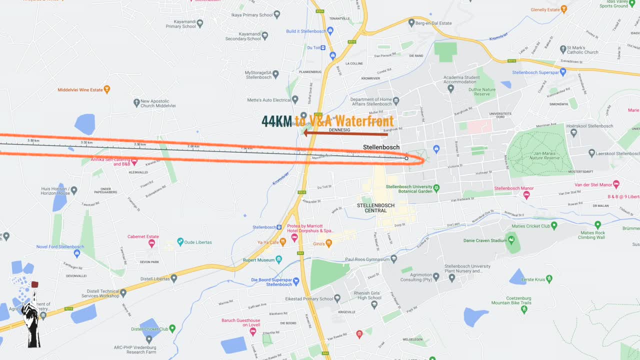 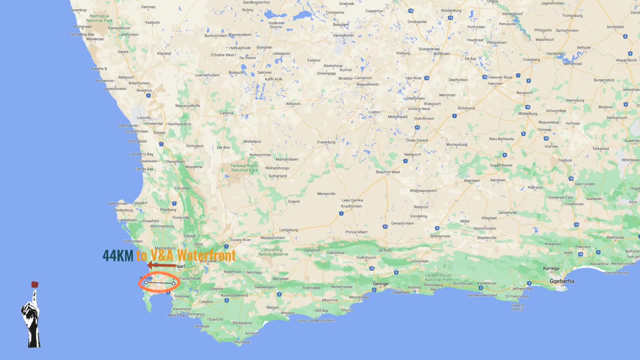 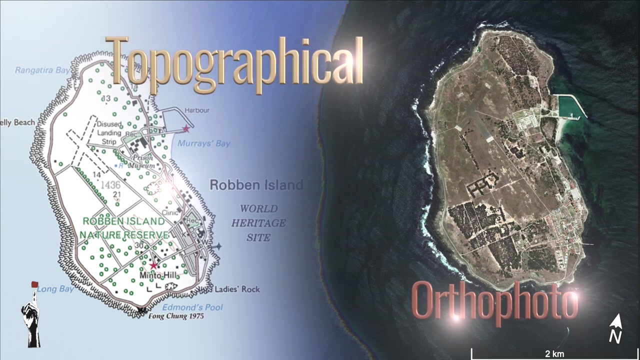 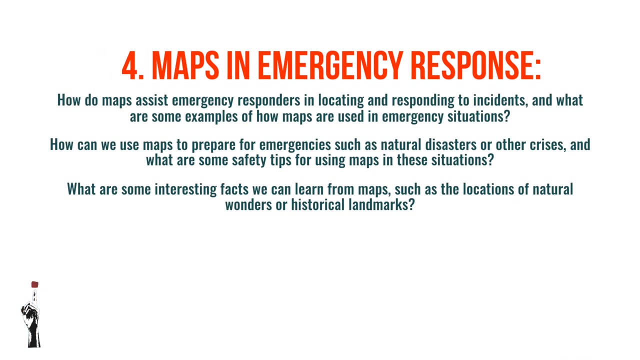 distance from the ground or in real life. Large scale maps show a small area in great detail, while small scale maps show a larger area with less detail. For example, we have orthophotos and topographical maps. as I've mentioned before, The orthophoto normally covers a demarcated area in a topographical map. 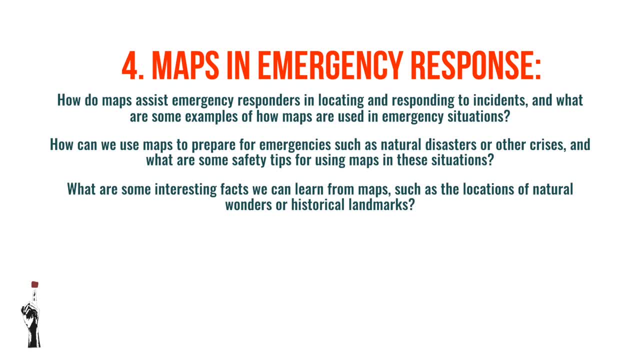 Now, if I put up the map date down on the map, then this map family sense looks like the manner in which the map is placed on the map. It might look like this and that …. And lastly, we have the concept of time zones. 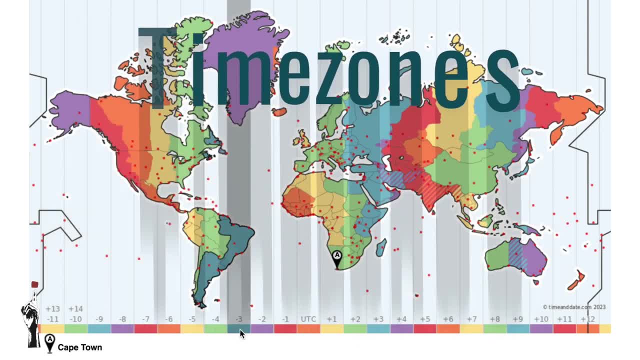 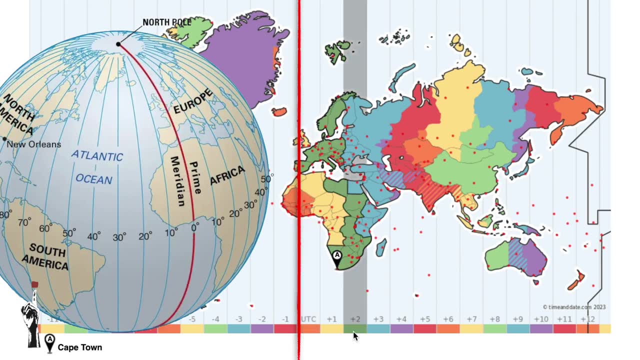 And lastly, we have the concept of time zones. Time starts at the Greenwich MeridianCHR, that is the zero行了 paradigm degrees line of longitude. There's a one-hour change in time for every 15 degrees At the 180 degrees line of longitude. we have the IDL, the 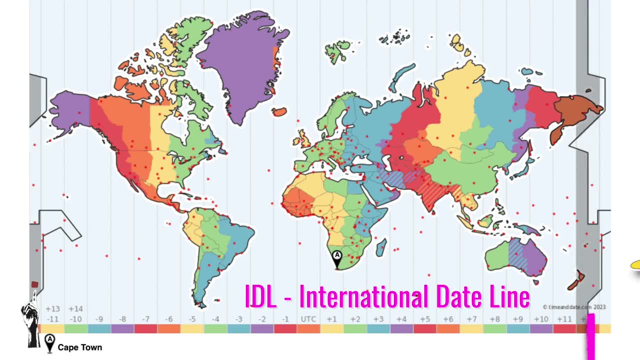 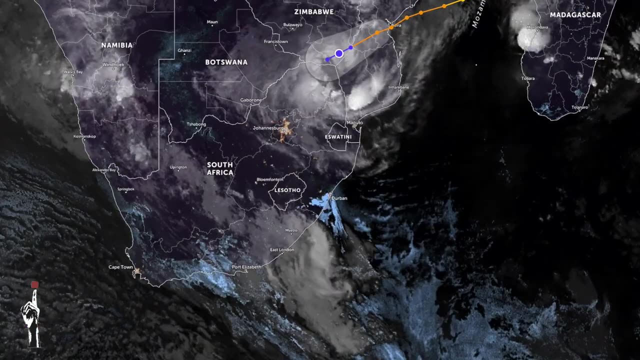 international date line. It's where the day changes. People traveling westward around the world must set their clocks back by one hour for every 15 degrees of longitude crossed, and forward by 24 hours upon crossing the international date line. Lastly, we have images taken from a satellite called satellite images, or 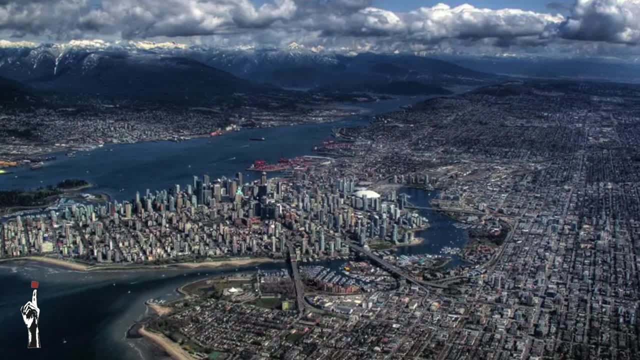 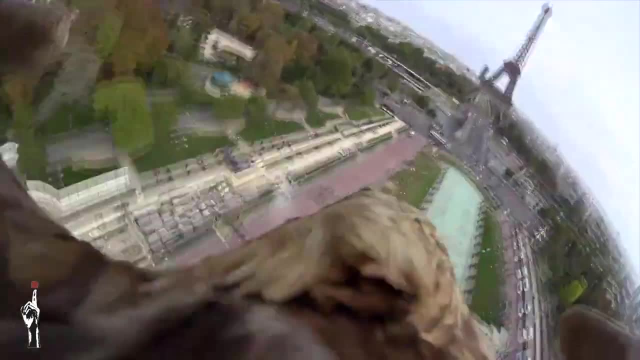 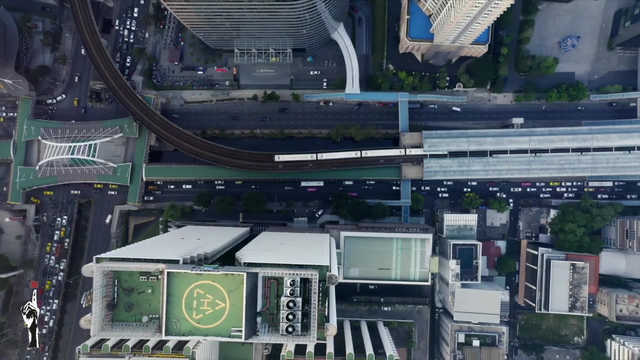 from an aeroplane, called aerial photos. We have two types of aerial photos: a vertical aerial photo or an oblique aerial photo. An oblique aerial photo is generally taken from an angle Think of a bird's eye view. A vertical one is taken from directly above the features mapped. These are: 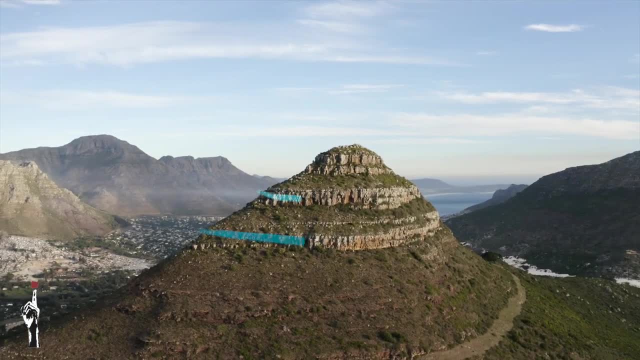 images of the earth's surface. These are images of the earth's surface. These are images of the earth's surface taken from space or from an aircraft, as I've said, and can be used to create maps and study the earth's surface in great detail. 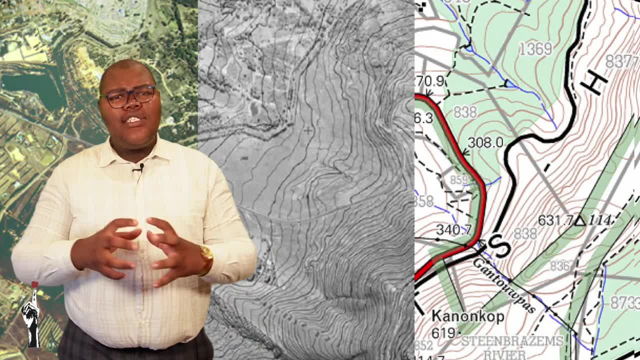 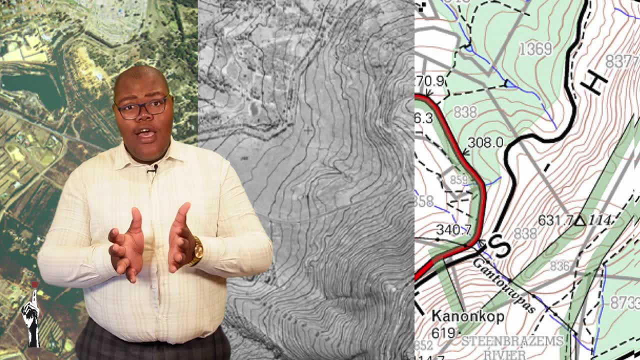 And so great eights and nines. we've currently reached the conclusion of our lesson. Now, this lesson was just to give you a quick overview of the most important types of maps. Of course, we're not saying these are all types of maps, but these are the ones you'll interact with as you go in your geography career. 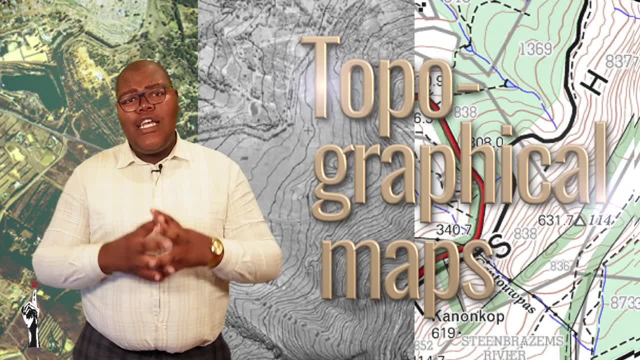 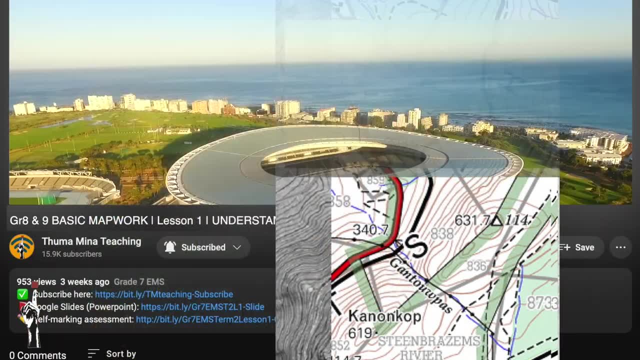 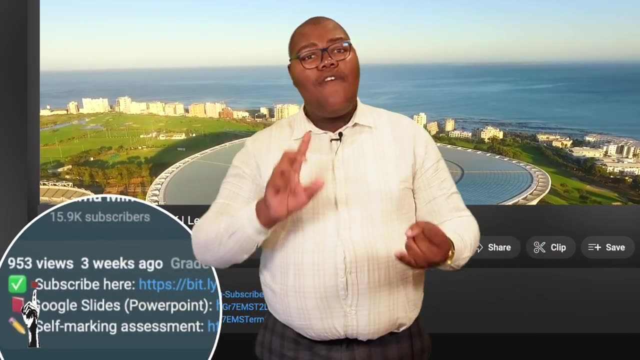 In our next lesson, we'll be zooming specifically into topographical maps, as these are maps that you'll be working with mostly this year and next year. Now, great eights and nines, remember to check the description of this video down below. Here you'll find a self marking assessment and Google slides. It is very. 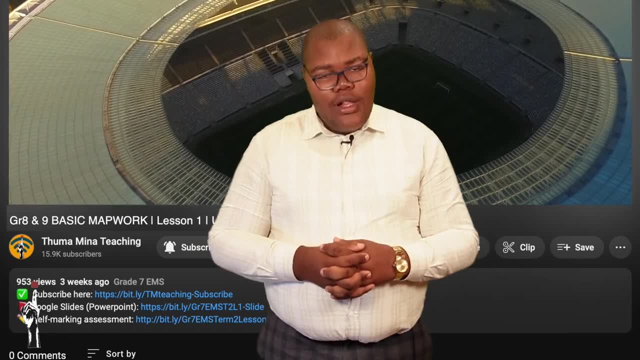 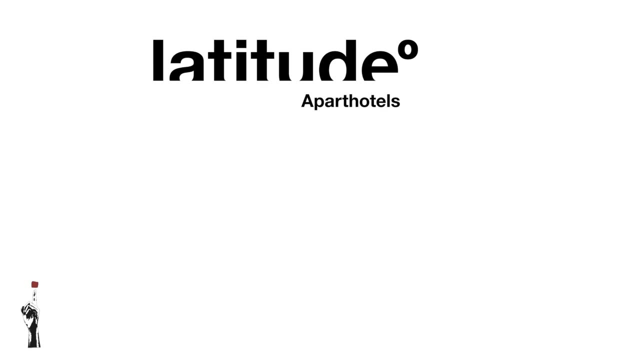 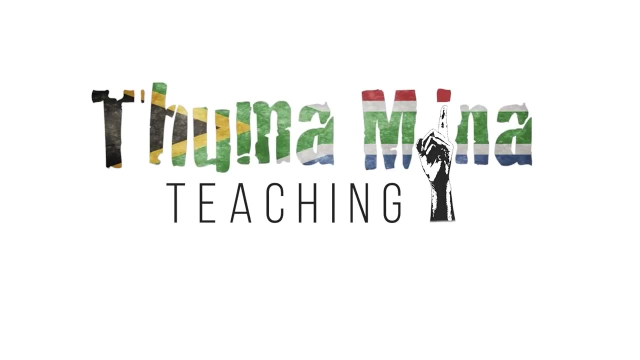 important to check your understanding, and this assessment will help you do just that. Thank you so much for watching. I wish you all the best for your map work and hope to see you next time. Music. 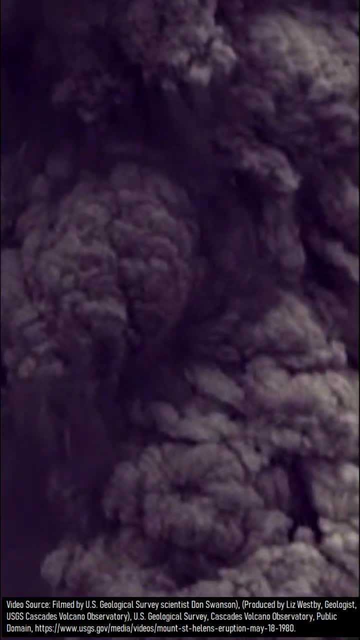 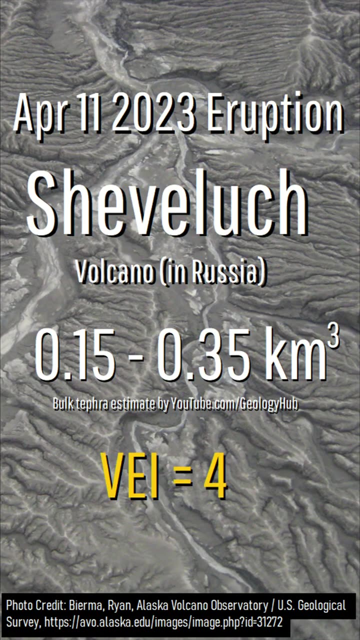 The April 11th 2023 eruption of the Shevlyush volcano in Russia was unusually large as, based on my own estimates, it probably ejected between 0.15 and 0.35 cubic kilometers of tephra. Yet 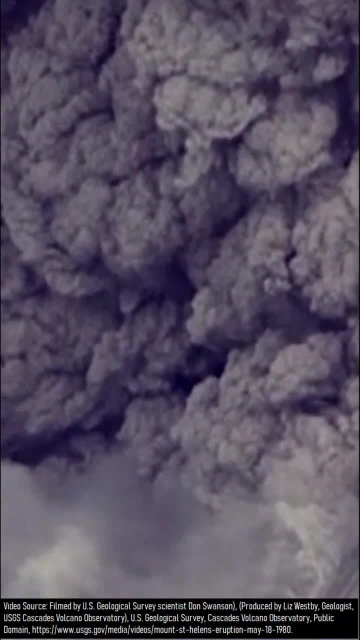 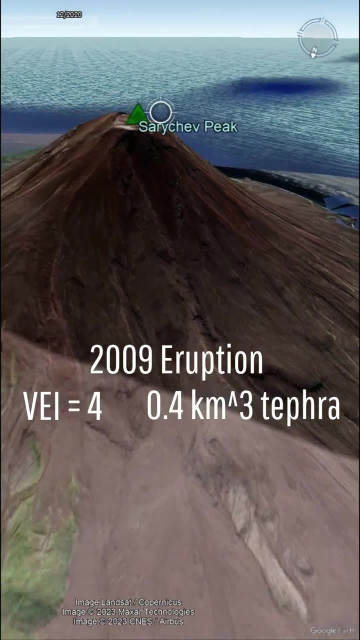 dozens of eruptions within Russia during the Holocene Epoch have been larger than this. Take, for example, the powerful eruption Serechev Peak produced in 2009, which ejected 0.4 cubic kilometers of bulk tephra, or the 1829 Klyuchevskoi eruption, which ejected 0.55 cubic kilometers of 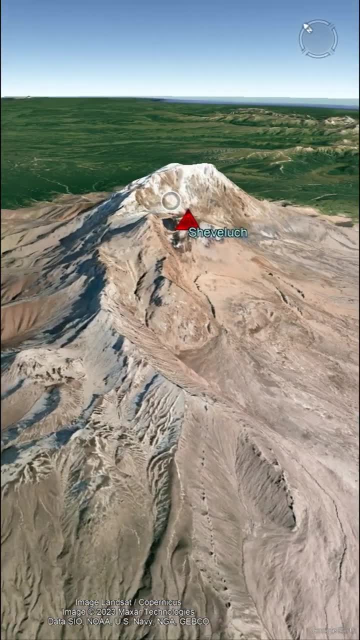 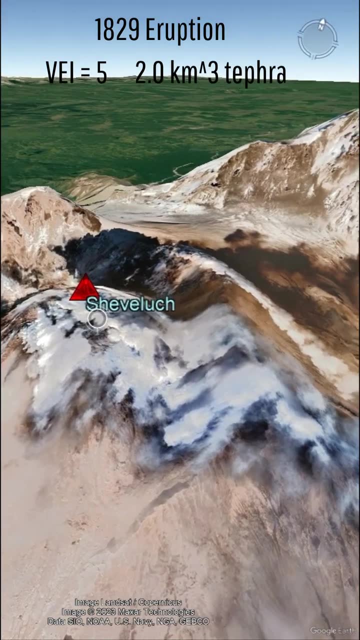 bulk tephra. Even comparing to prior Shevlyush eruptions, this was smaller than its 1964 eruption, which was smaller than its 780 BCE eruption, which was smaller than its 1854 eruption. Yet all of these eruptions were smaller than the 610 eruption of Opala, 5922 BCE eruption of. 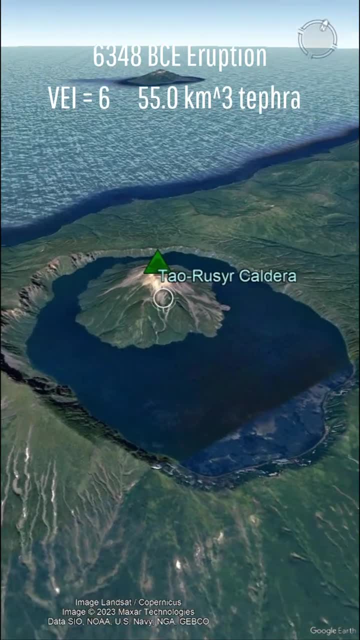 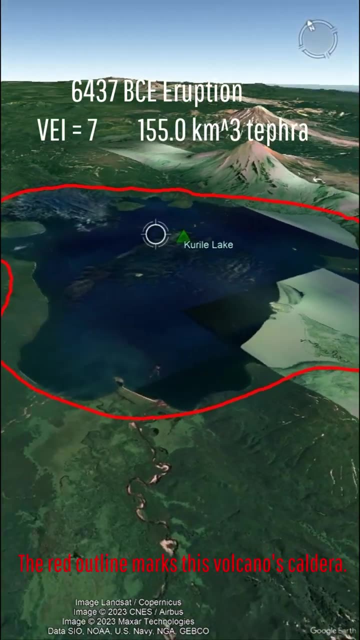 Khangar, which formed a caldera 6348 BCE. eruption of the Tauruzer caldera, or Livinaya, passed in 8685 BCE. Yet the largest volcanic eruption Russia has produced during this period was a 6437 eruption of the Tauruzer caldera, which formed a caldera. 6348 BCE. eruption of the Tauruzer.